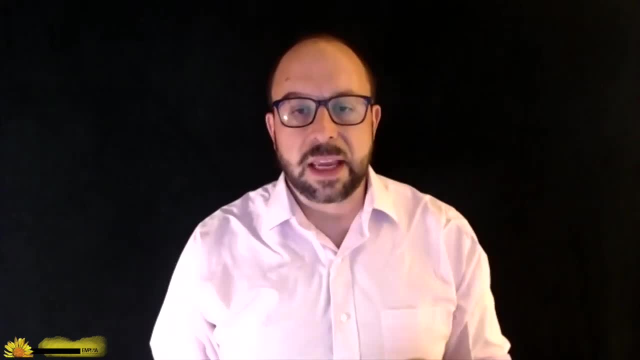 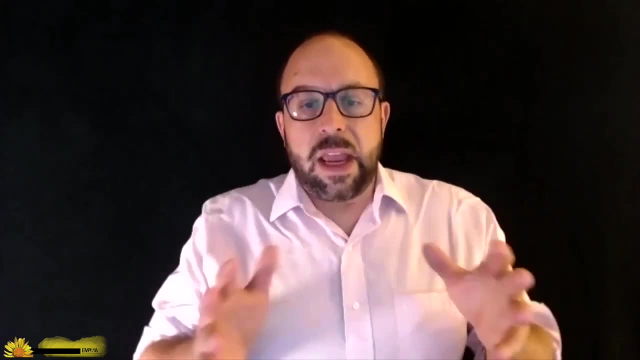 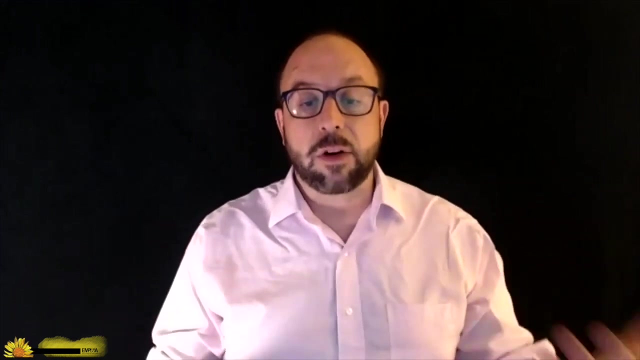 important. The first most common mistake is a failure to search the records before filing. Searching the records is extremely important. First of all, a search in general of more than just the USPTO records is very important when creating and launching a new program. So if you're looking for a new program, you're looking for a new program. 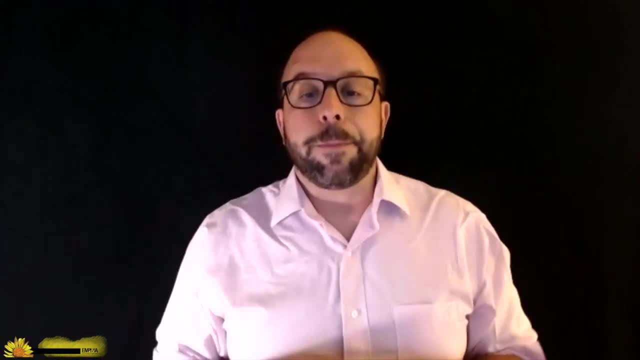 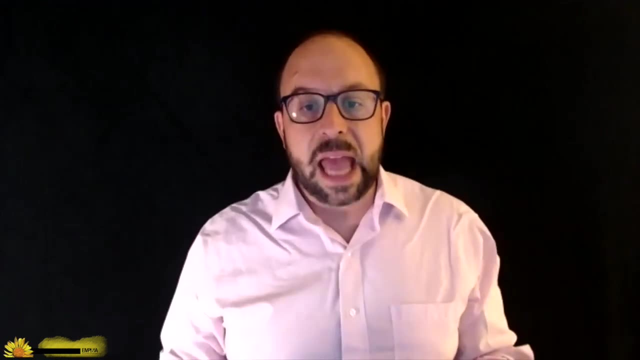 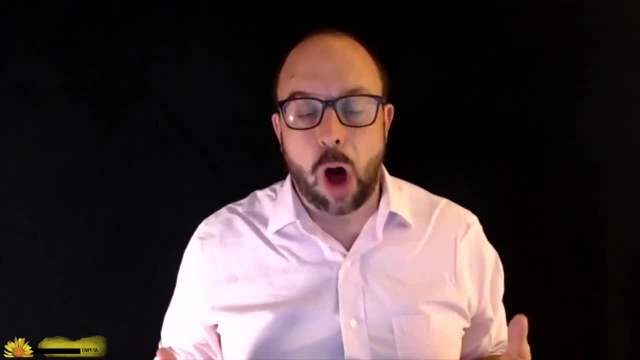 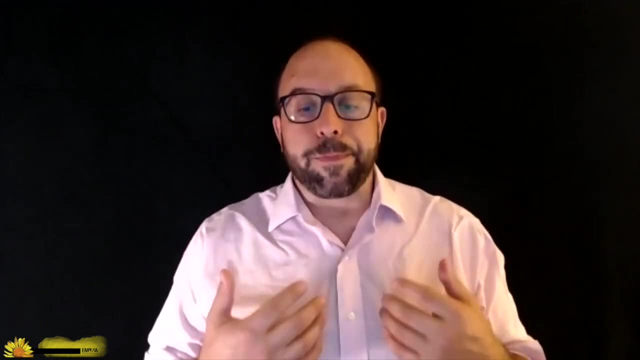 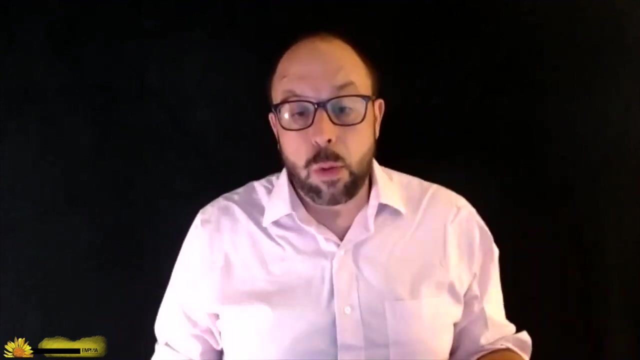 else might be out there. that is a potential obstacle or conflict, because that might affect our strategy, our goals and our drafting of the application. So it's very important to search beforehand. It's also possible you find something that you didn't know about. that is like a clear conflict. 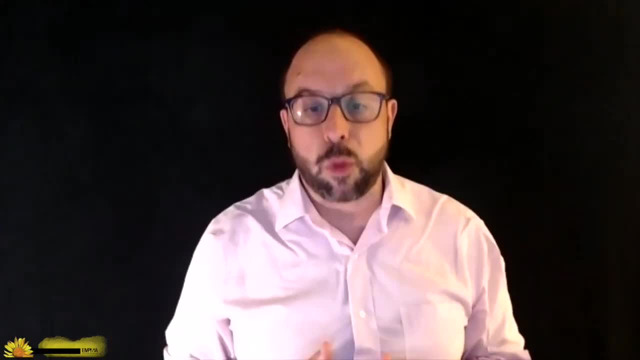 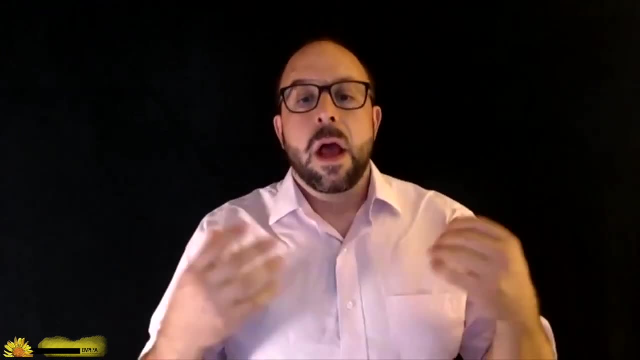 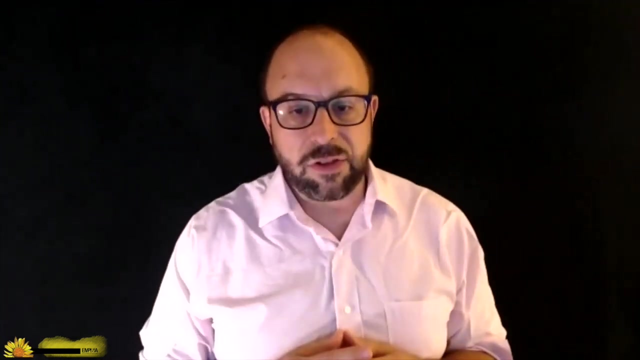 that, would you know, have even greater ramifications beyond just the application. But at a minimum you want to search the USPTO before filing. The second important thing that I often see a failure to comply with is the specimens of use in the application. It is. 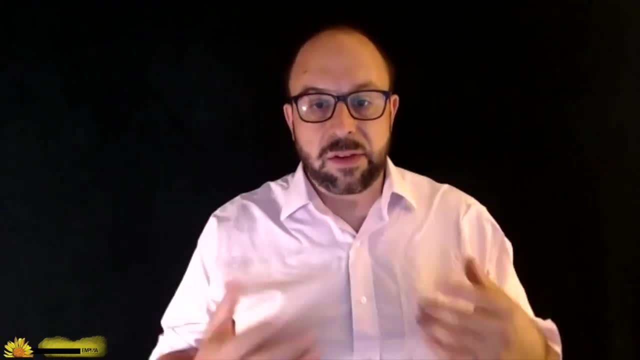 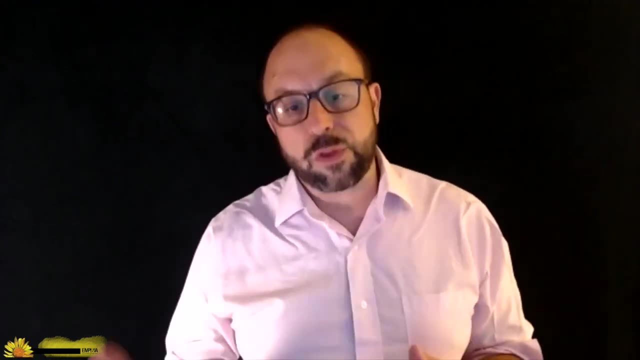 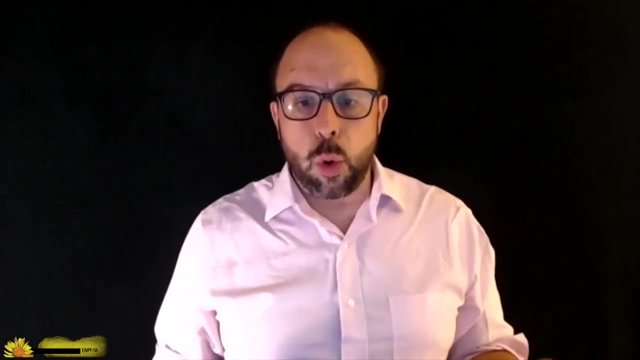 important to submit the right types of evidence for the trademark. Now this depends on where the application is, Whether the application is for goods or for services. there are different types of evidence or specimens that are acceptable, And there are new rules for submitting certain. 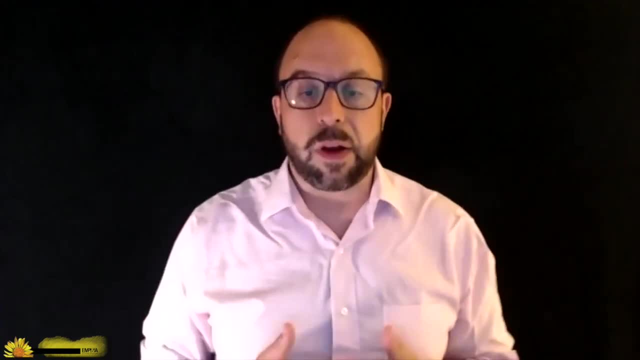 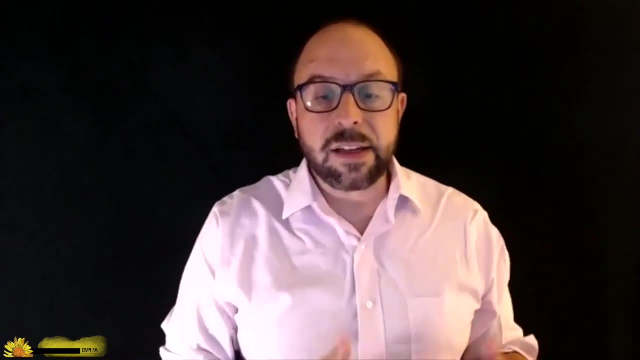 types of specimens, like screenshots and procedures, that you must comply with. So it's very important to make sure you get the specimens correct. Even if you're filing a intent to use application, you will eventually have to file the evidence of use, And it's a second important element. 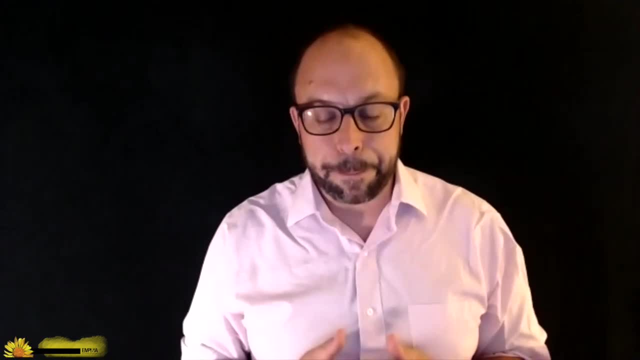 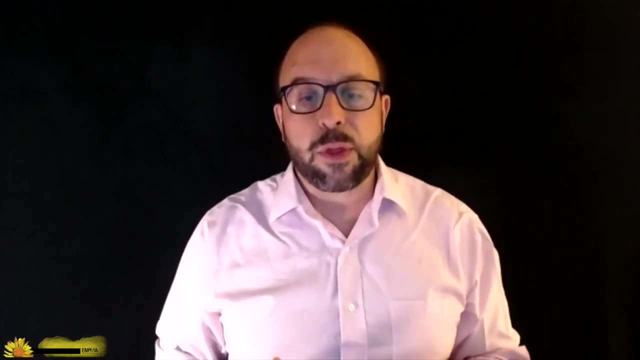 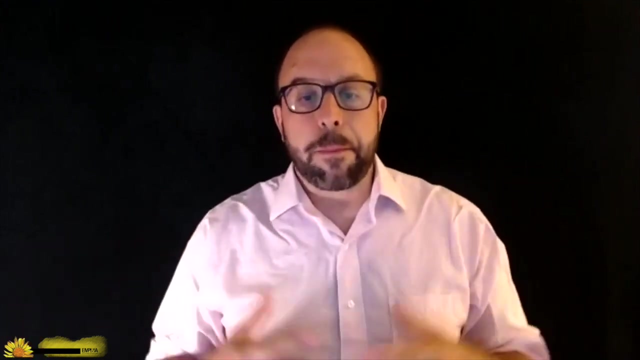 of the application that I often see People make mistakes on. The third and final one is the descriptions of goods and services And the description- I say it for third because it really ties the first two together- The mark and the evidence must match, along with the description of products and services.